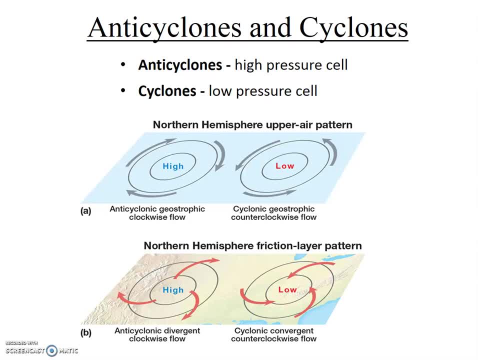 We now have a basic understanding of wind direction around high and low pressure cells at the Earth's surface and at higher altitudes. These high and low pressure systems also have names: High pressure cells are called anticyclones and low pressure cells are called cyclones. Let's review the 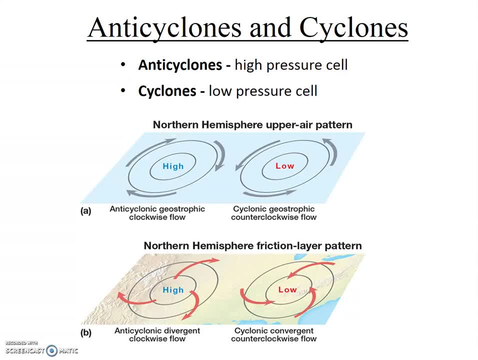 diagrams you drew. You drew six diagrams, but on this page we have omitted the hypothetical pressure gradient, only diagrams. So here the top diagrams represent upper atmosphere flow and the bottom diagrams represent surface winds. Now we know to call the high pressure cell diagrams on the left of this. 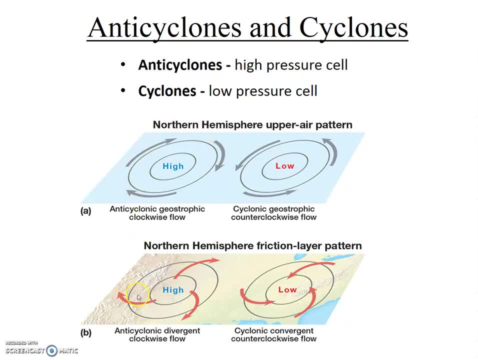 diagram here Anticyclones And the low pressure diagrams here represent cyclones. Let's review the diagrams In a high pressure system or an anticyclone in the upper atmosphere. we're only dealing with the pressure gradient and the Coriolis. 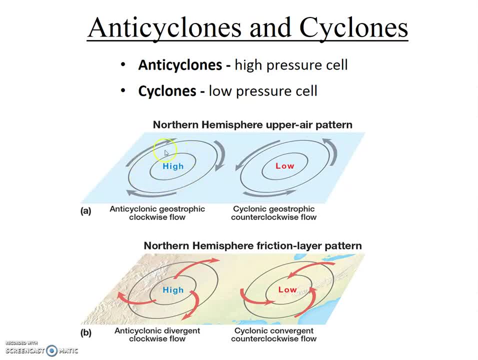 effect and the resulting winds are what we call clockwise geostrophic flow. Down closer to the surface of the Earth, friction is involved, which reduces the Coriolis effect and essentially the pressure gradient overwhelms the Coriolis effect and we have what's called divergent clockwise flow. There's 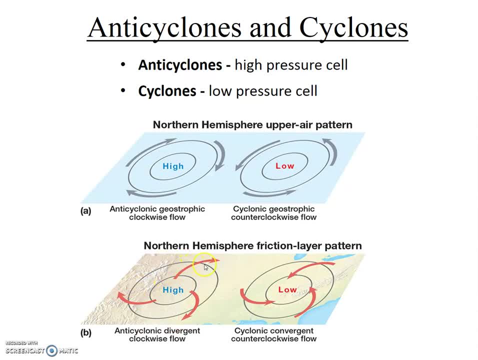 still a clockwise nature to it. but the air is also diverging. In a low pressure cell or cyclone, we have in the upper atmosphere simply the pressure gradient and the Coriolis effect and they balance each other out and we end up with counterclockwise geostrophic flow In the lower atmosphere. friction plays a. 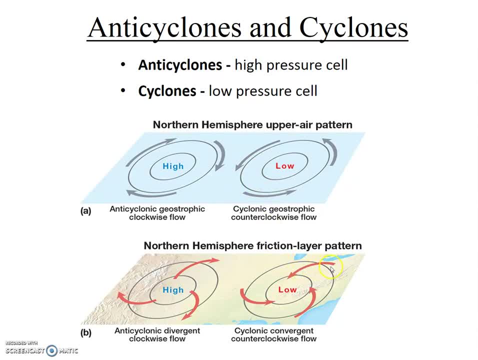 role, The Coriolis effect is reduced and we have still counterclockwise flow. but now, since the pressure gradient overwhelms the Coriolis effect, we have counterclockwise convergent flow. When I was learning this material, I found it helpful to remember that in the 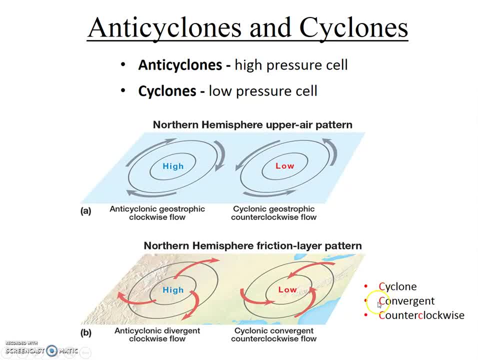 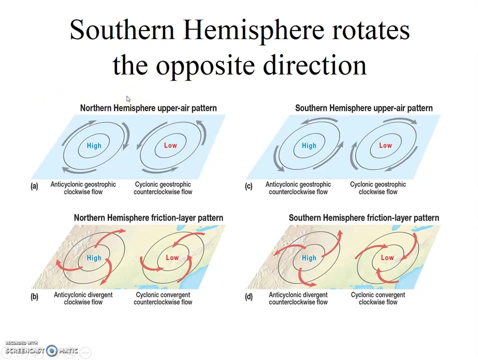 cyclones which start with the C. you have all the C words. It's convergent, counterclockwise flow, A lot of C's. Thus far, we have focused on the northern hemisphere and we will continue to do so, but the southern hemisphere flow. 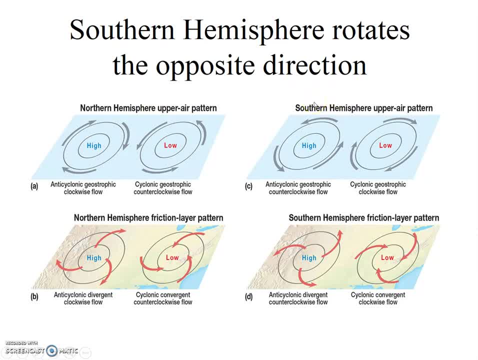 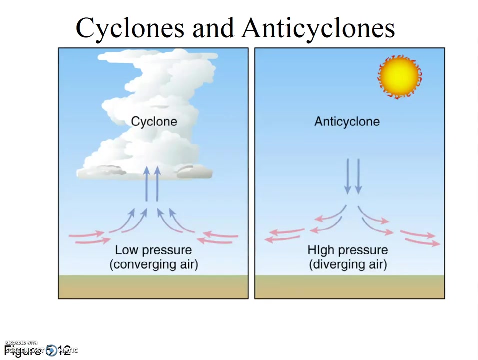 patterns simply change the rotation direction. The upper atmosphere winds are still geostrophic and the lower atmosphere winds are still divergent or convergent, depending on which type of pressure cell exists. Only the direction changes. Next we're going to add one more component to our model. We will add the 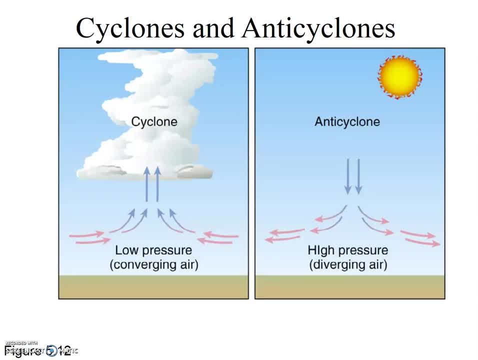 vertical component within the center of the pressure cells. First let's consider the high pressure system, the anticyclonic system. The air at the surface is diverging. But where does this diverging air come from? Air is entering from the center above. Thus the vertical movement in the center of an anticyclone is 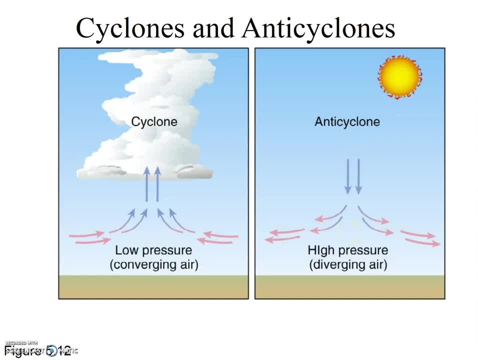 downward. Notably in the center of any pressure cell, high or low, there is very little horizontal air movement, very little wind. The primary motion in the center of one of these cells is down for anticyclones and up for cyclones As we. 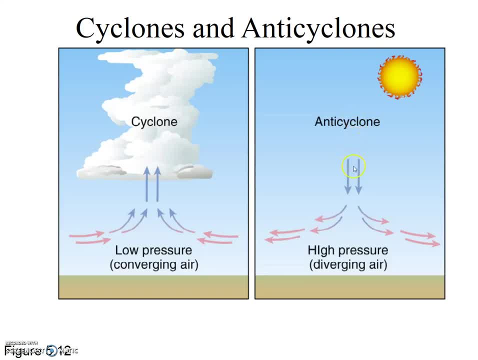 see here in anticyclones, the cool air is descending in the middle and then diverging outward at the surface. This descending air actually helps create the high pressure. Also importantly, next week we're going to learn that rising air is needed in order to form clouds. Thus, since 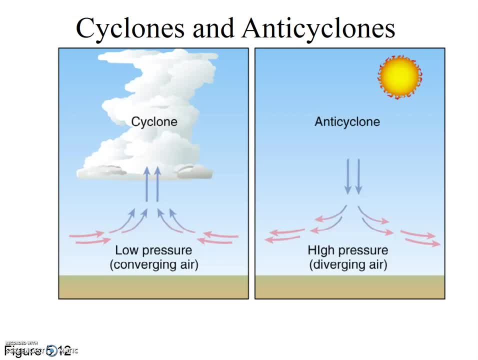 anticyclones have descending air. they do not produce clouds or rain. Rather, as shown here, they are characterized by beautiful, blue, cloudless skies. Next, let's consider the low pressure system. the cyclones Air is converging towards the center, But where does this diverging air come from? The vertical movement in the center of an anticyclone is 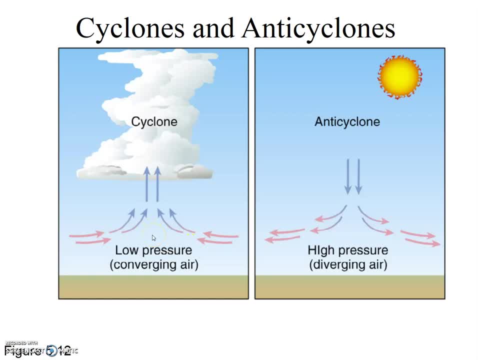 upward. Where does this converging air go? It has to go somewhere. Air leaves the cell by rising upward. Thus the vertical motion in a cyclones in a low-pressure cell is upward Again, just like in high-pressure cells. the center of a low-pressure cell has little horizontal air movement very. 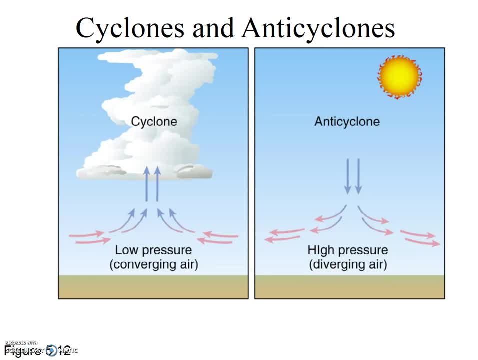 little wind, The primary motion is upward for cyclones, just as it was downward for anticyclones. In cyclones, warm air is rising in the middle and indeed this rising air helps create the low pressure and since rising air is needed to form, 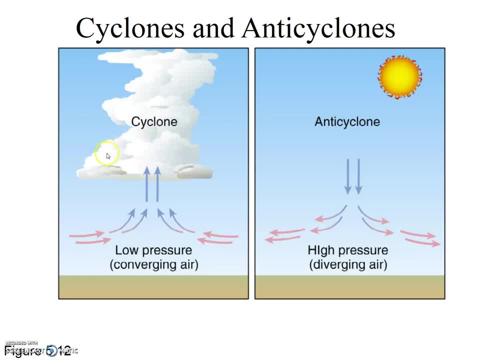 clouds. cyclones are excellent cloud producers and are characterized by cloudy skies. Indeed, that's another C we can add to our memory: aid Cyclones have counterclockwise convergent flow in the lower atmosphere and then, as the air rises, clouds form. Pause the video and talk your way through each of these. 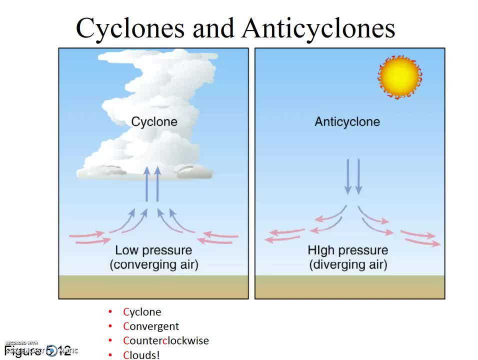 diagrams again. In a low-pressure cell or cyclone, air converges with counterclockwise rotation in the northern hemisphere and the air rises to form clouds. In a high-pressure cell or an anticyclone, the cool air descends and diverges, and 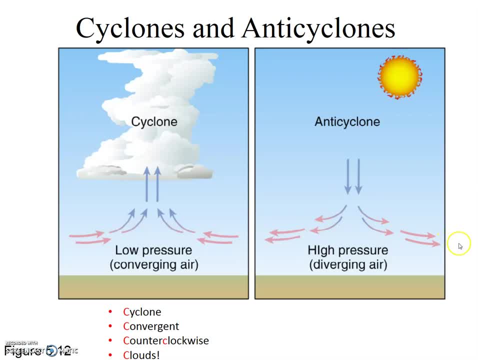 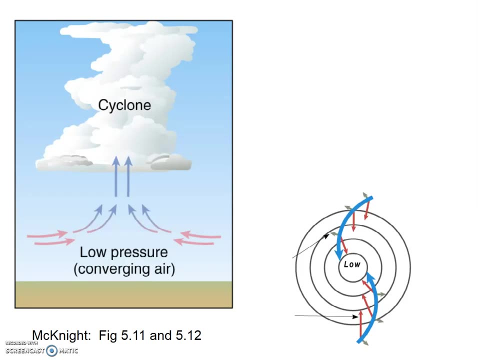 the skies are clear And in the northern hemisphere that would be clockwise diverging air for the surface winds. One more time looking at a cyclone: At the surface we have counterclockwise convergent air going towards the center and in the center we have rising air which rises up to form clouds In the 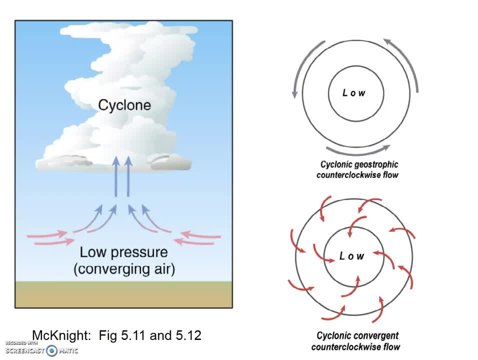 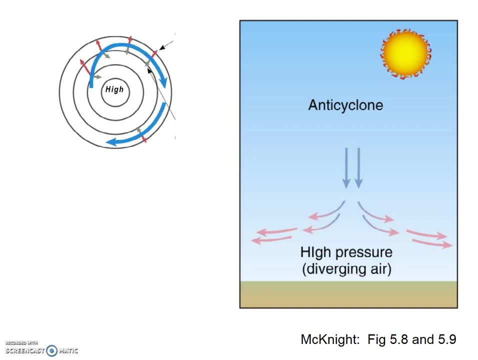 upper atmosphere we don't have the influence of friction, so the motion is counterclockwise, geostrophic flow. In an anticyclone we have air descending in the center and that upper atmosphere air is moving clockwise in a geostrophic manner. As the air descends it diverges outward. for clockwise divergent flow We don't. 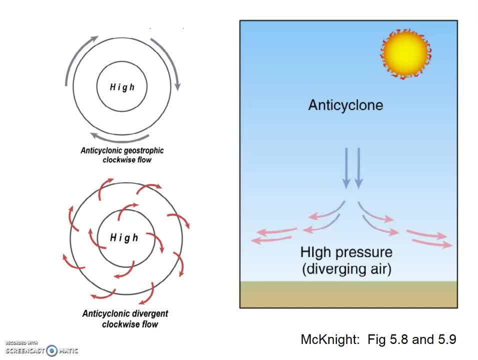 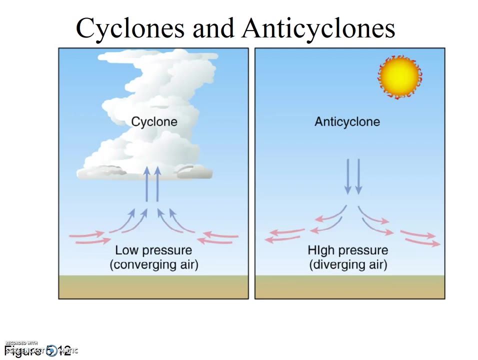 expect there to be clouds in a high-pressure anticyclone, because the air is descending and, in general, you need rising air to form clouds. Okay, now let's take it one step further. Where would you expect to find cyclonic air flow At the 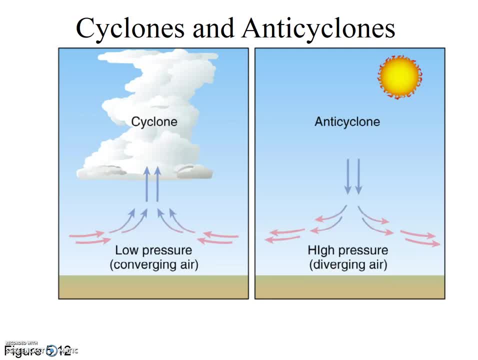 equator or at the poles? How about anticyclonic air flow? Again, pause the video and think about that. Which one of these diagrams would be typical at the equator and which one would be typical at the poles? Where would you expect rising air and why would it rise? 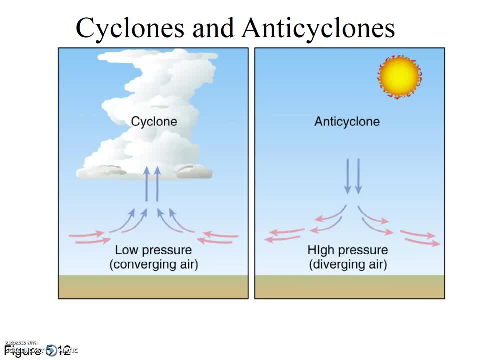 Okay, hopefully, you said you would find a low pressure cell or a cyclone near the equator and an anticyclone would be near the poles. Why? Well, near the equator the air is warm, and the warm air expands, becomes less dense and rises. thus. 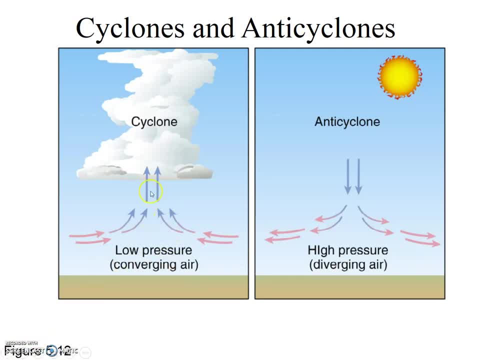 forming a low-pressure cell and creating clouds. That fits nicely with our understanding from last week that the equatorial regions do not have the highest temperatures in the world due to frequent cloud cover. At the poles, the opposite is true: We have cool descending air, forming a high-pressure system and 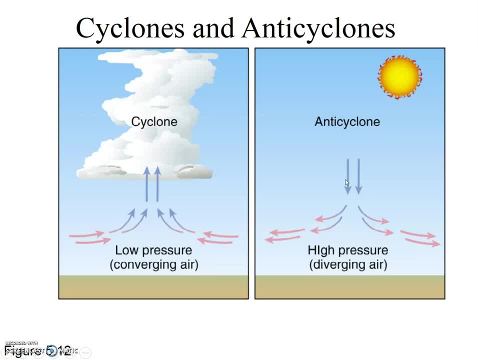 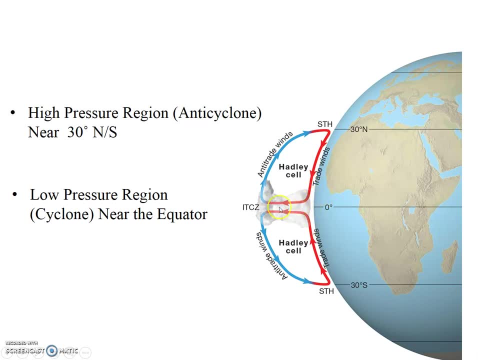 clear skies. This diagram shows a low pressure cell near the equator. the converging air rises and forms clouds. We'll see shortly that the rising air actually starts to move poleward at high altitudes and eventually at approximately 30 degrees north and south. 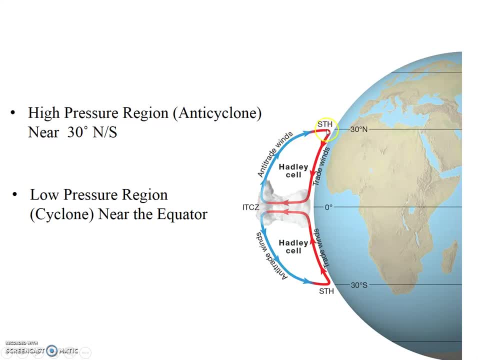 the air is cooled enough that it starts to descend again, creating a high pressure cell right around 30 degrees north and 30 degrees south. Indeed, right around 30 degrees north and 30 degrees south, there's a fairly consistent region of high pressure with cloudless skies. This is where we find the world's 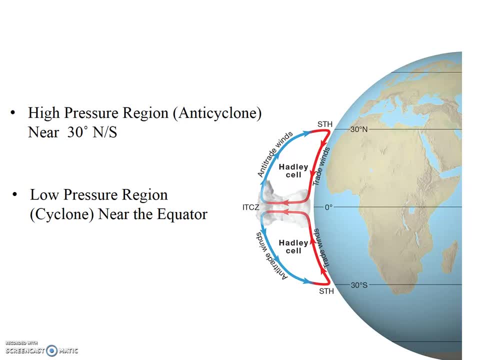 highest temperatures in the interiors of the continents and, additionally, because there are no clouds, or very few clouds. this is also the location of many of the world's deserts. Pretty cool, eh, Check it out. most of the world's deserts are somewhere near 30 degrees north or south. All right, let's use what we know. 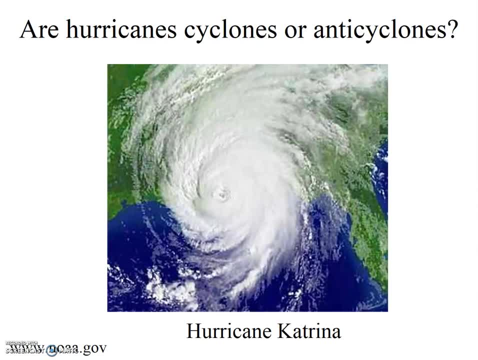 about cyclones and anticyclones. to determine if hurricanes are cyclones or anticyclones, Check out this remote sensed image of Hurricane Katrina. Are the surface winds converging or diverging? Are the winds clockwise or counterclockwise? Pause the. 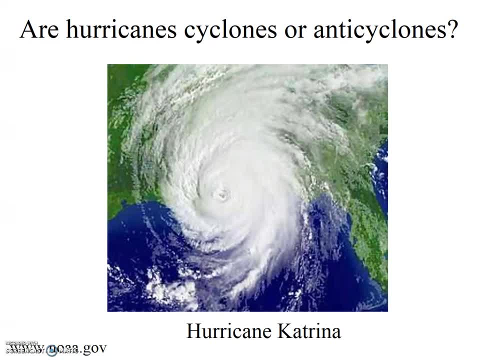 video and check it out, Hopefully. you said that the winds were converging and counterclockwise. That's correct. So does that make this a cyclone or an anticyclone With convergent, counterclockwise winds? indeed, that makes this a cyclone. Actually, the clouds also. 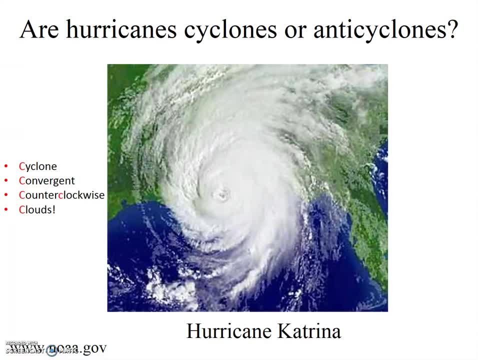 give it away. What would an anticyclone look like on an aerial photo? You wouldn't see the rotation much at all, as there would be no clouds. Also consider what a hurricane would look like in the southern hemisphere. It would still have the cyclonic air flow, so still have the converging air that ascends in the 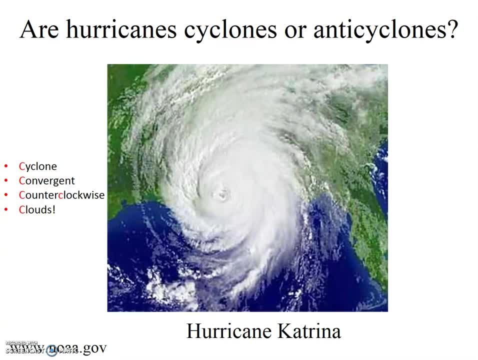 middle. However, the direction would be different. in the southern hemisphere Cyclones, so hurricanes would flow clockwise. Keeping that in mind, do you think hurricanes generally ever cross the equator If they flow, if the air flow is clockwise in the Southern Hemisphere and counterclockwise in the Northern Hemisphere? 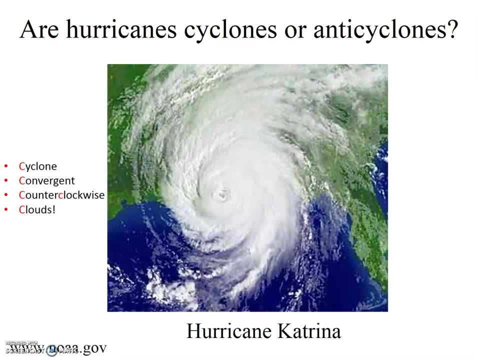 it seems unlikely that a hurricane could easily cross the equator. All right, so we now have a pretty good understanding of pressure and wind. We understand the three factors that affect wind direction, and we know something about both lower atmosphere and upper atmosphere winds in both high pressure and low pressure systems.